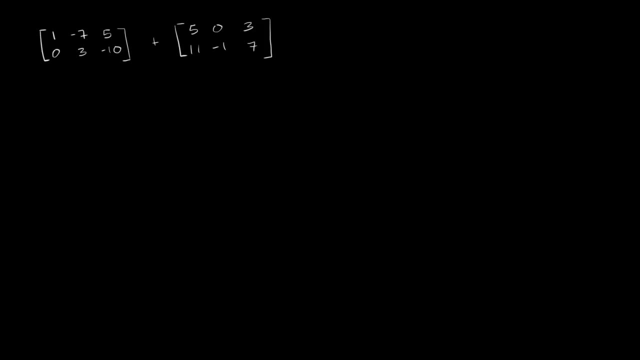 Let's think about how we can define matrix addition, And mathematicians could have chosen any of an arbitrary number of ways to define addition, But they've picked a way to define addition that seems one to make sense And it also has nice properties that 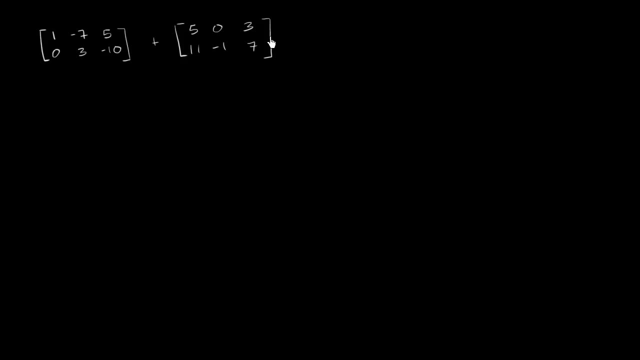 allow us to do interesting things with matrices later on. So if you were one of these mathematicians who are first defining how matrices should be added, how would you define adding this first matrix over here to the second one? Well, the most common sense thing. 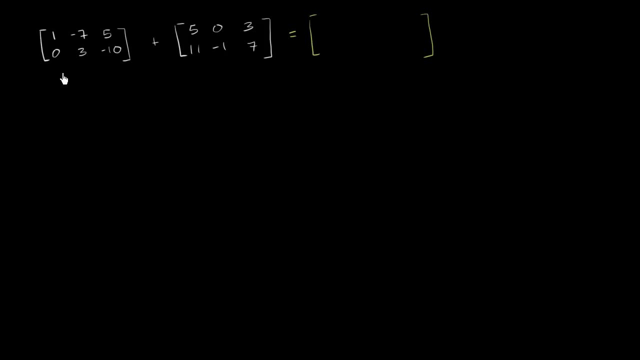 that might have jumped out at you, especially because these two matrices have the same dimensions. this is a 2 by 3 matrix, has two rows and three columns. This is also a 2 by 3 matrix: two rows and three columns. 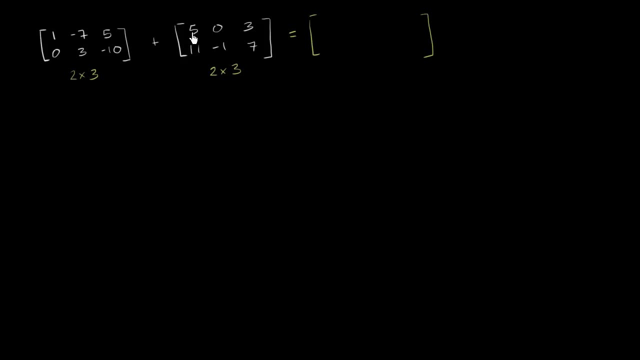 is to just add the corresponding entries. And if that was your intuition, then you had the same intuition as the mathematical mainstream that the addition of matrices should literally just be adding the corresponding entries. So in this situation we add 1 plus 5. 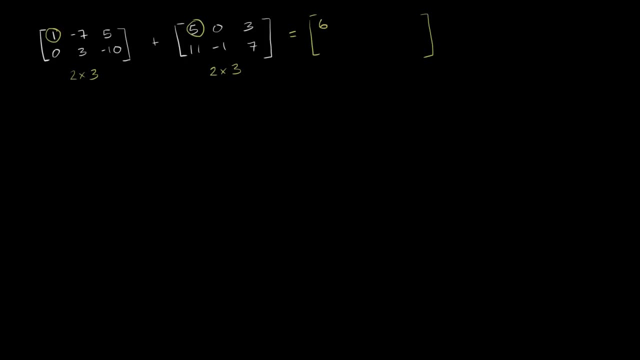 to get the corresponding entries. So you can add the same entry in the sum, which is 6.. You can add negative 7 plus 0 to get negative 7.. You can add 5 plus 3 to get 8.. You can add- and I'm running out of colors here- 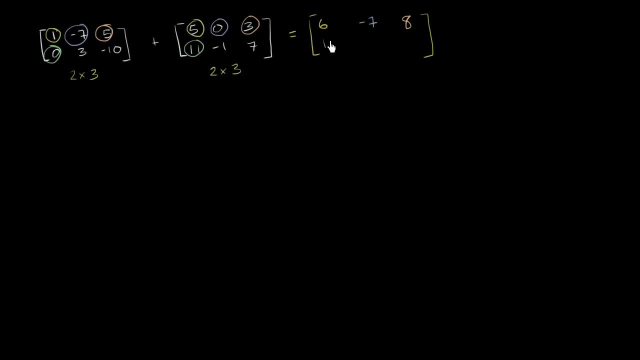 you could add 0 plus 11 to get 11.. You can add 3 to negative, 1 to get 2.. And you could add, And you could add negative 10 plus 7 to get negative 3.. And if you see this definition of matrix addition. 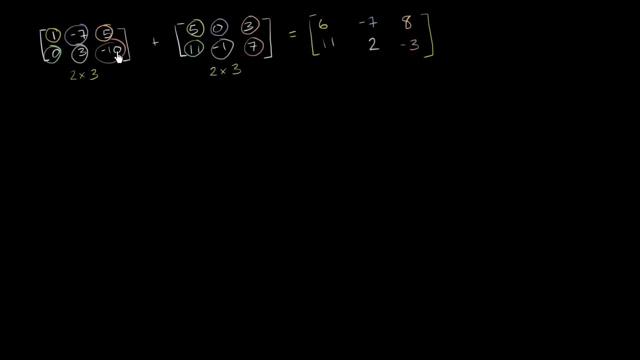 you see that it actually does not matter in what order that we actually add these matrices. I could have done this the other way around. If I did this the other way around, let me copy and paste this. So, if I were to add this matrix, so let me copy and let. 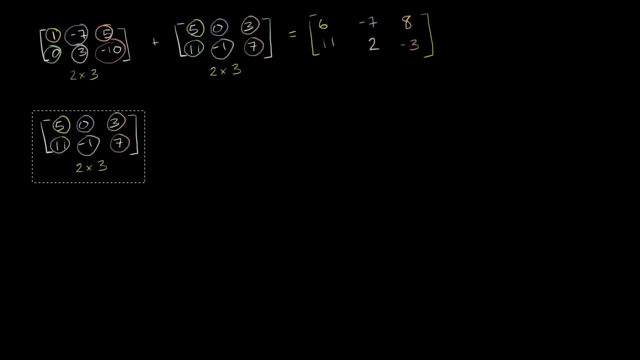 me paste it If I were to add it this way, that matrix to let me copy and paste the other one to this matrix. So copy and paste. If I were to go this way, you'll see that the order in which I'm adding the matrices. 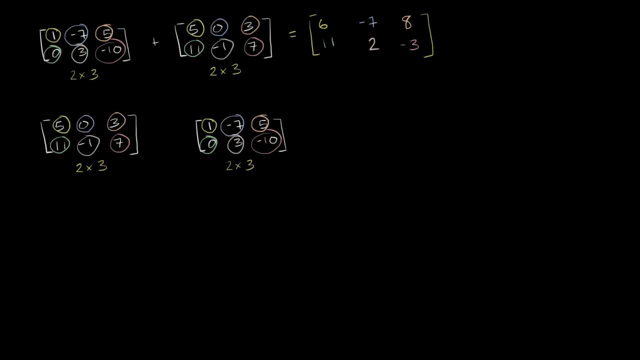 does not matter. So this is just like adding numbers: a plus b is the same thing as b plus a. What we'll see is that this won't be true for every matrix operation that we study. In particular, this will not be true for matrix multiplication. 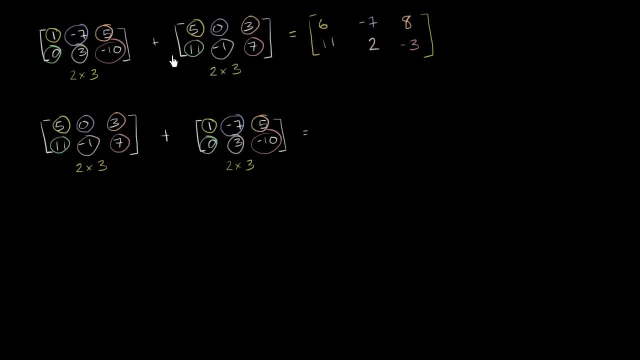 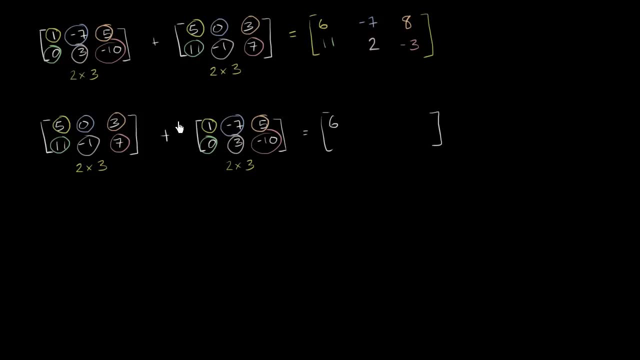 We get the same result, because 1 plus 5 is the same thing as 5 plus 1.. Here we add 0 plus negative 7.. You get negative 7.. So you're going to get the exact same thing as we got up here. 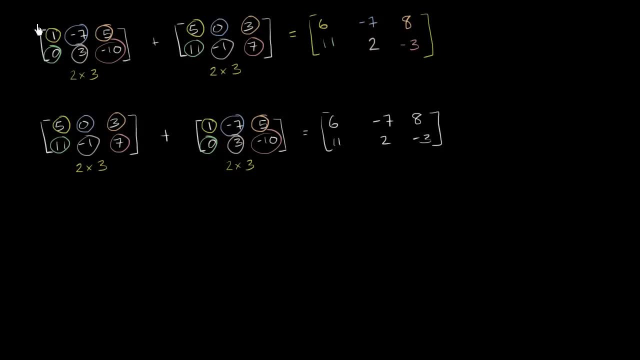 So when you're adding matrices, if you were to call this matrix right over here matrix A, which we normally denote with a capital bolded letter, and you call this matrix right over here matrix B, then we take the sum of a plus b, which is this thing, right. 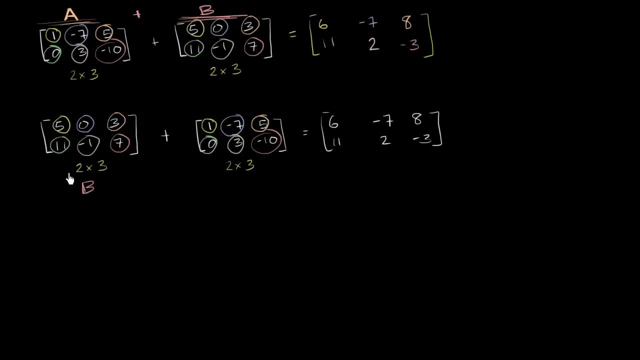 over here and we see it's the exact same thing. It's the same thing as matrix B plus matrix A. Now let me ask you an interesting question: What if I wanted to subtract matrices? So let's once again think about matrices that have the same dimensions. 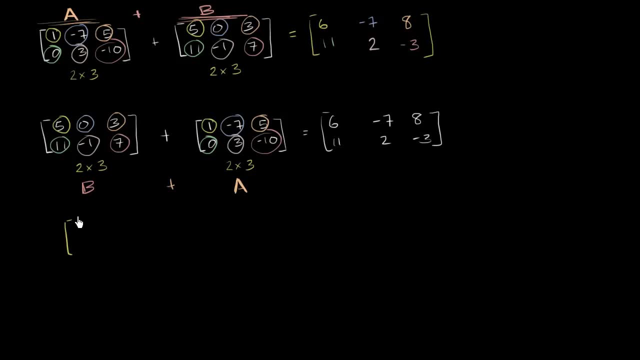 So let's say I'm going to have two 2 by 2 matrices. So let's say it's 0, 1,, 3,, 2.. And from that I want to subtract negative 1,, 3,, 0, and 5.. 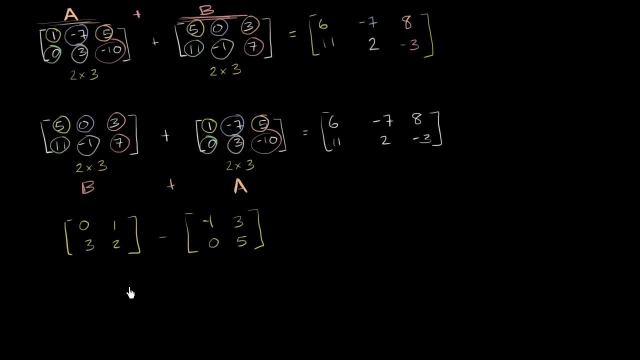 So you might say, well, maybe we just subtract corresponding entries, And that, indeed, is how you can define matrix subtraction. In fact, you don't even have to define matrix subtraction. You can let this fall out of what we did with scalar multiplication and matrix. 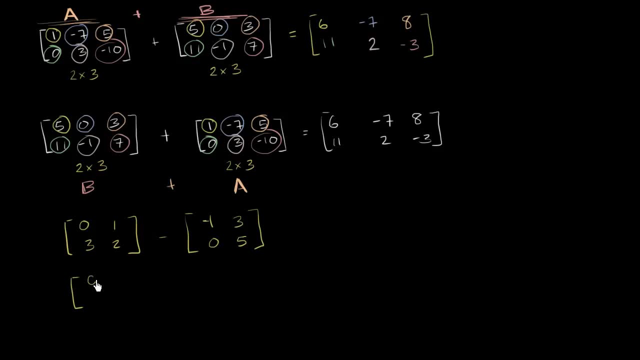 addition, We could view this as the exact same thing as taking 0,, 1,, 3,, 2, and to that we add negative 1 times negative: 1, 3,, 0,, 5.. And if you work out the math, you're. 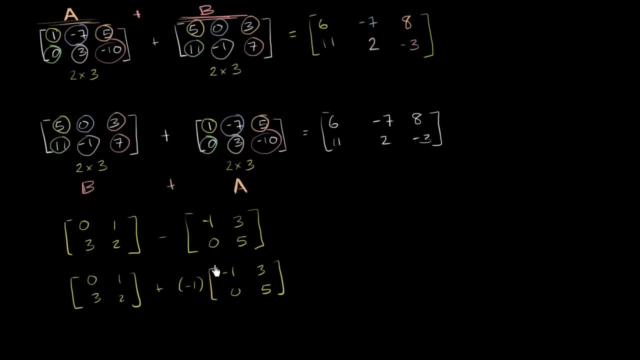 going to get the exact same result as just subtracting the corresponding terms, So this is going to be 0 minus negative, 1 is positive, 1.. 1 minus 3 is negative, 2.. 3 minus 0 is 3..